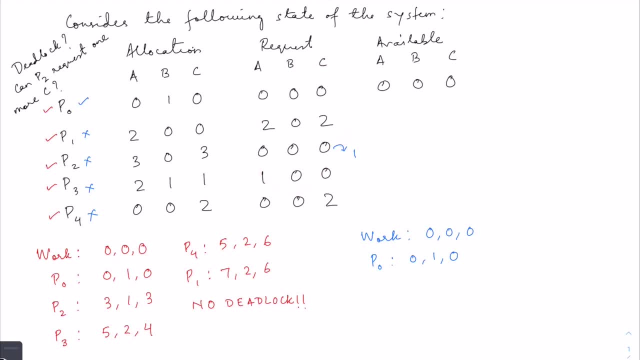 And what is the request matrix? So here for P1 we have 2 0, 2. that means P1 at this point of time has requested 2 more instances of A, nothing of B and 2 more instances of C, And available vector is the number of all the instances free in the system available. 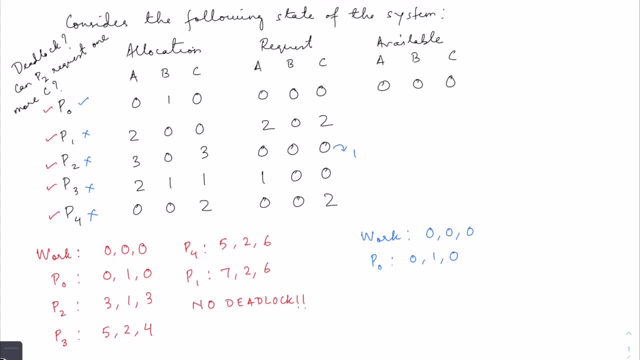 for use. So let's run the deadlock detection algorithm to see if this system is currently in a deadlocked state. So to begin with, we will first see if any of the allocations are completely 0, and then we can go ahead and mark the finish variable for those processes. 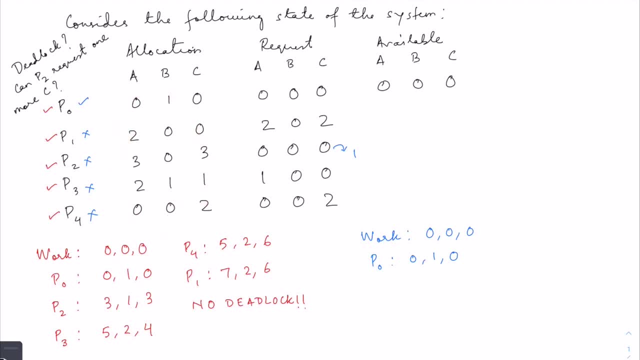 to, true, But looks like none of them are completely 0. So we have a 1 over here, we have a 2 over here, here we have a 2, so none of them are completely 0. So we cannot mark any of the. 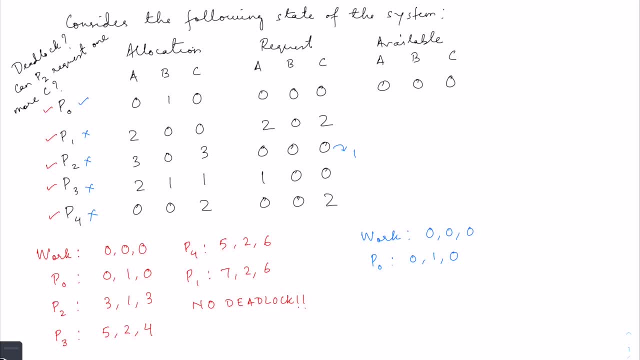 finish variables to true at this point of time. So just imagine, none of these red tick marks are there. all of them are not finished at this point of time. So we take the work variable to be the available vector at this point of time and we will look. 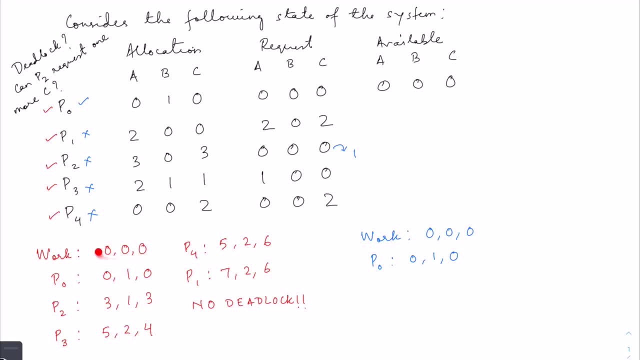 at a process whose request can be satisfied with whatever we have in the work pool over here. So we have all 0's. so let us look at a process whose request is 0 and P0 happens to be that process, So we mark P0 as done. 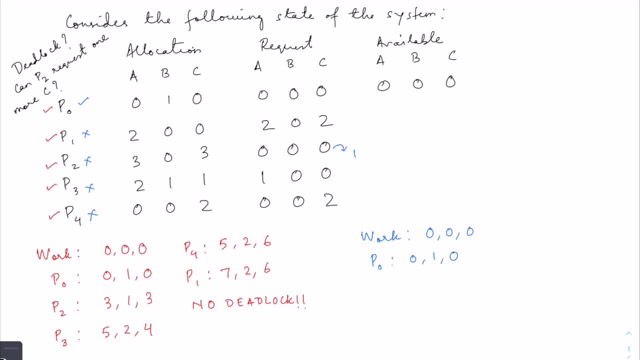 So we put a red tick mark over here, we take its allocation and we add it back to the workpool over here. so from 0 0 0 and we add 0 1 0 to that and it becomes 0 1 0 here let's look. 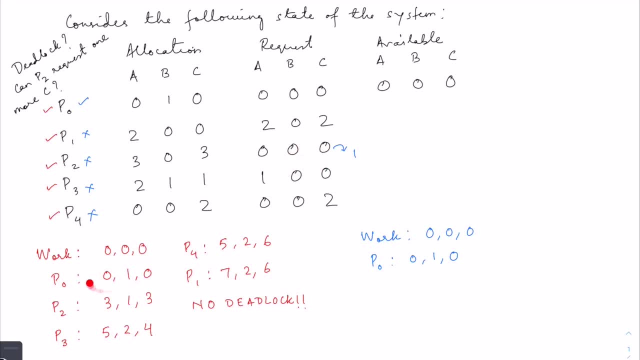 at another process whose request can be satisfied with whatever we have in the work pool. that is 0 1 0, so let's go for process P2, because its request is also 0 0 0, ignore this one. that is for the second step of this problem, and so we mark P2 as done, as finished and 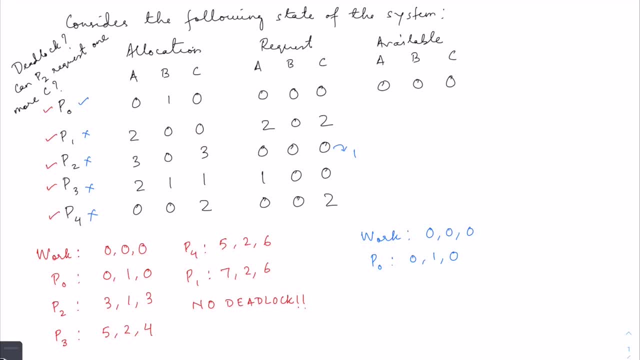 we take its allocation and we add it to the work pool of 0 1 0 and we get 3 1 3. now let's go to P3, because its request is 1 0, 0 and that can be satisfied by 3 1 3. so we mark: 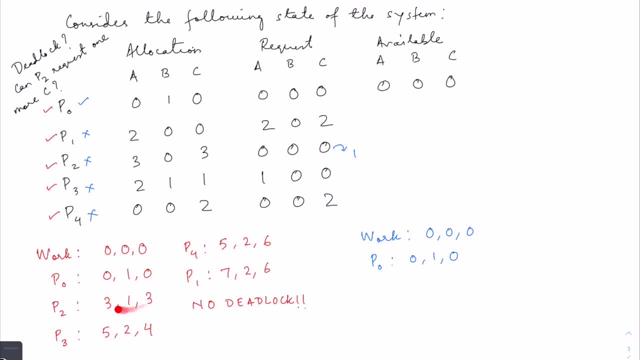 P3 as done. we take its allocation and we add it to the work pool and we get 5, 2, 4. then we mark P4 as done, then we mark P1 as done in a similar way. in the end we see all the processes can finish, so there is no deadlock. 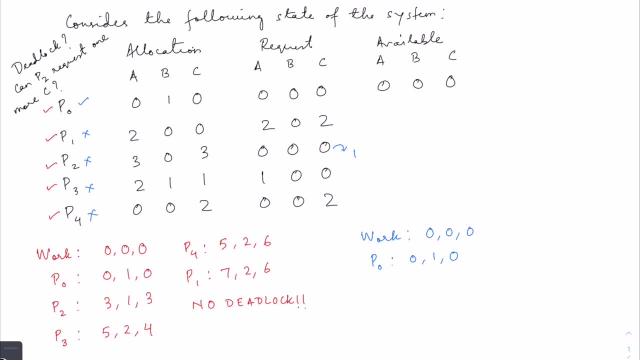 So we have finished all the processes and now we are going to go to the next step of this problem. the second part of the question tells us that P2 requests one more C, one more instance of resource type C, and if P2 does that, will the system enter a deadlocked state? 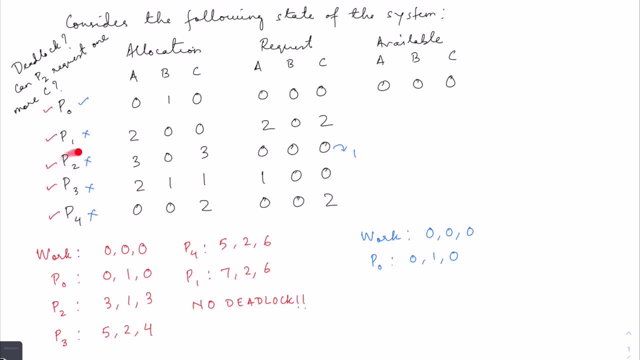 so what I am going to do is change the request of P2 for resource type C from 0 to 1 and we will try to rerun the deadlock detection algorithm. so, once again, I will take the request to 0 0 0, because available is 0 0 0 at this point of time, and we will look at a process. 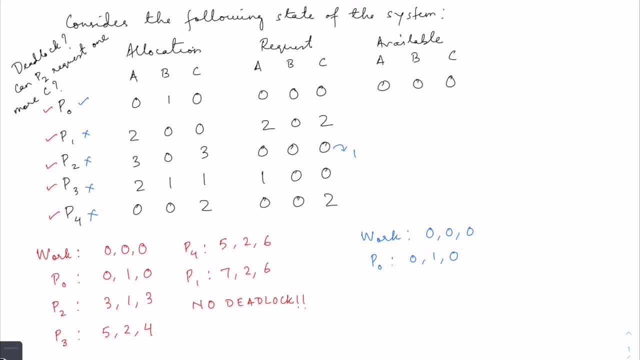 whose request can be satisfied with the current work pool we have over here. so again, we will go to P0, because its request is still 0 0 0. P2 is not 0 0 0, it is 0 0 1 right now. so 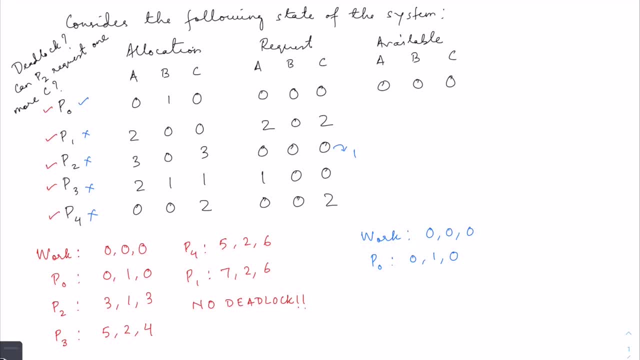 P0 is the only process we can go to. we put a blue tick mark which signifies that it has finished execution. we will take its allocation, add it back to the work pool. so from 0 0- 0 it has now changed to 0 1 0. now lets find a process whose request can be satisfied with. 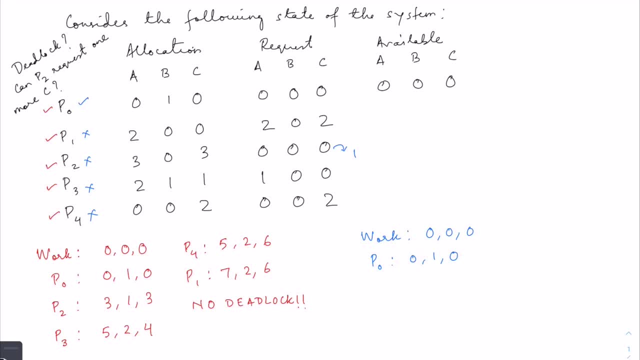 whatever we have in the work pool over here. so P0 is done. can P1 be done? 2 0 2? no, cannot be handled by 0 1 0. can P2 be done? 0 0, 1? no, 0 1 0 cannot handle 0 0, 1. because in this case, 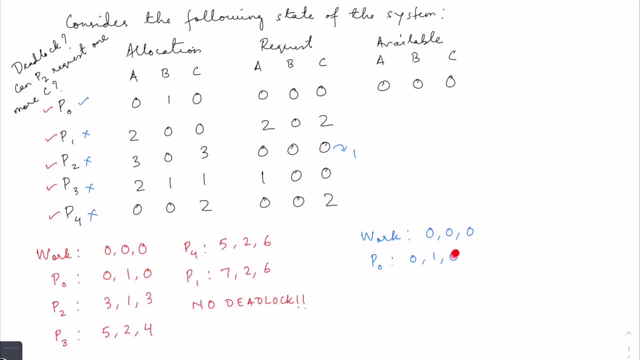 in the work pool we dont have any type C resources. P3: 1 0 0. can 0 1 0 handle that? no, because in the work pool we dont have any type A resources, can the request of P4, that is, 0 0 2, be handled?